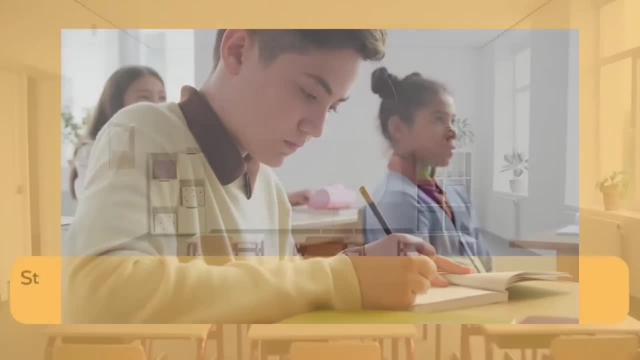 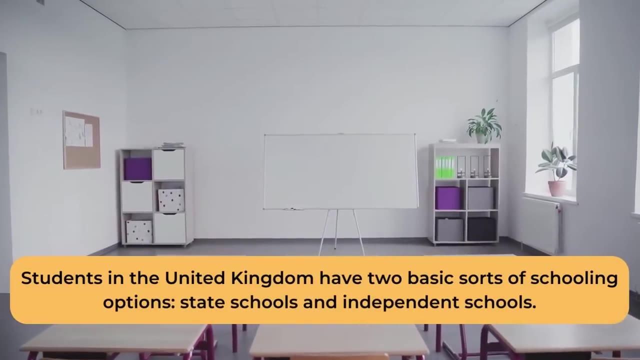 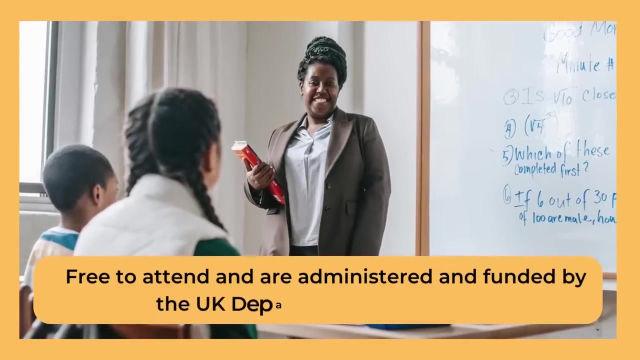 chosen subjects to receive a GCSE. Students in the United Kingdom have two basic sorts of schooling options: state schools and independent schools. Over 90% of British students attend state schools, which are free to attend and are administered and funded by the UK Department of Education. 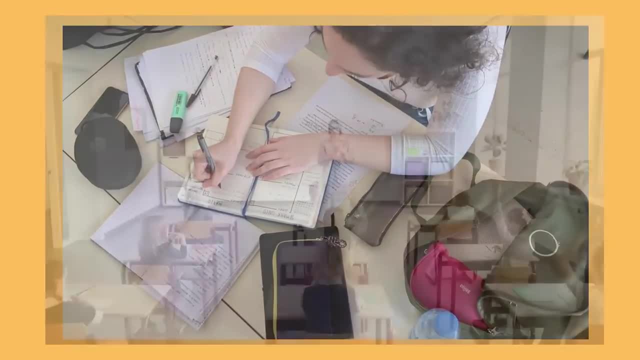 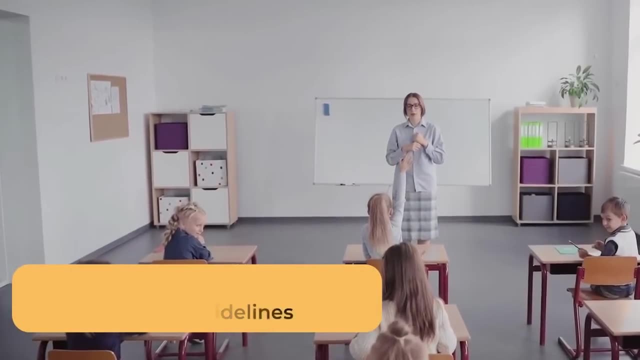 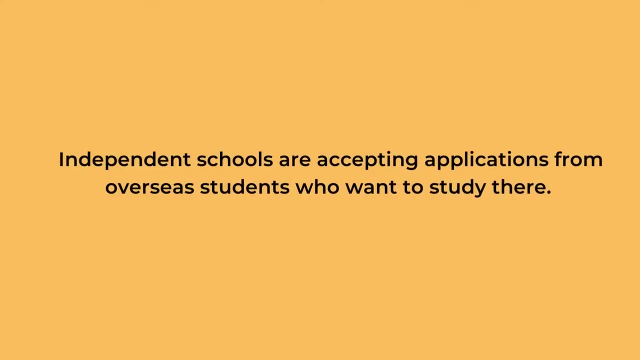 Independent schools that charge tuition are also available to students. Although these schools are not run by the government, they must nonetheless follow the government's educational guidelines. Independent schools are accepting applications from overseas students who want to study there, Except for dependent children accompanying an. 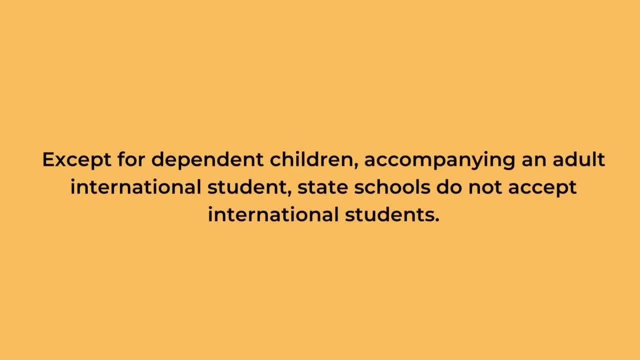 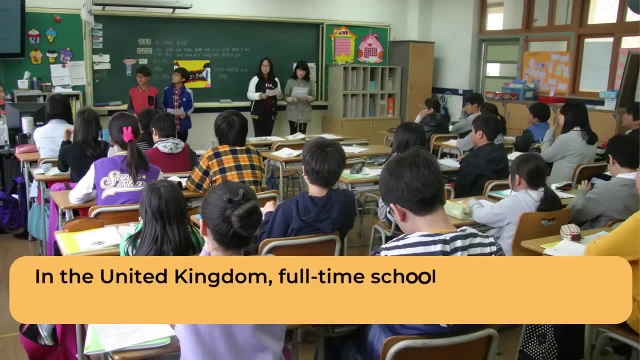 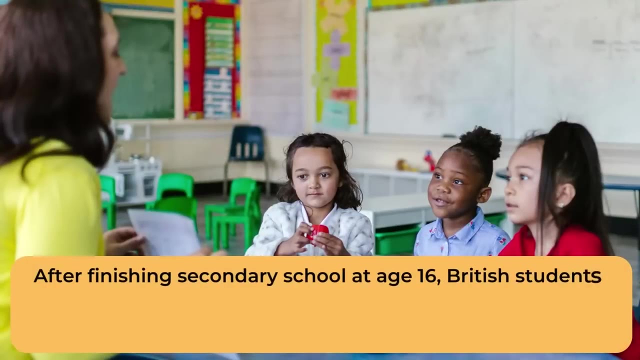 adult international student state schools do not accept international students. Further Education In the United Kingdom, full-time schooling is required until the age of 18.. After finishing secondary school at age 16, British students attend a Further Education institution for two years, referred to in their educational path as Year 12 and Year 13.. 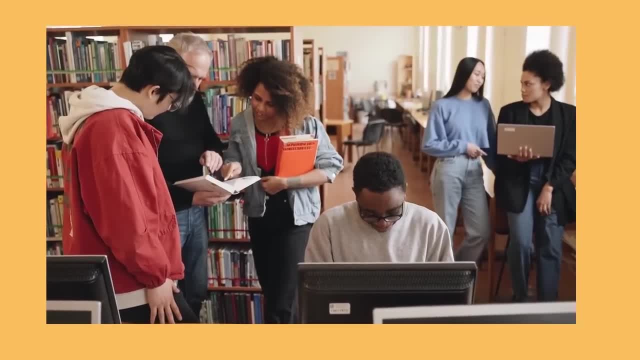 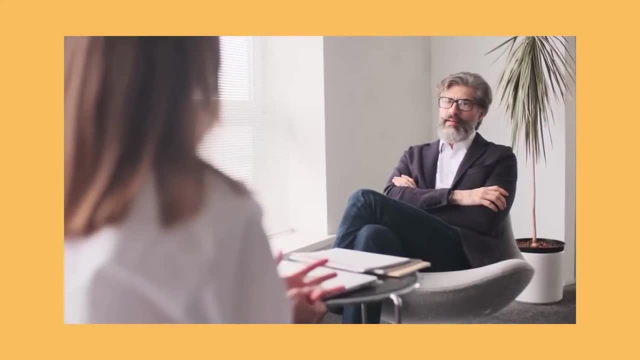 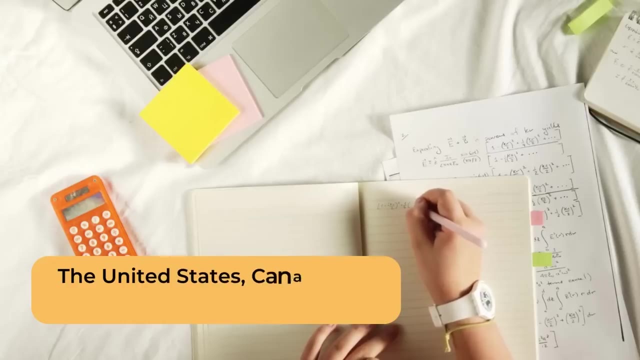 After graduation, the student can either pursue academic degrees that are necessary for university admission or obtain occupational credentials that will allow them to enter the job market right away. Admission is determined on a student's GCSE results. In the United States, Canada and many other countries, Further Education is comparable to the final years of secondary. 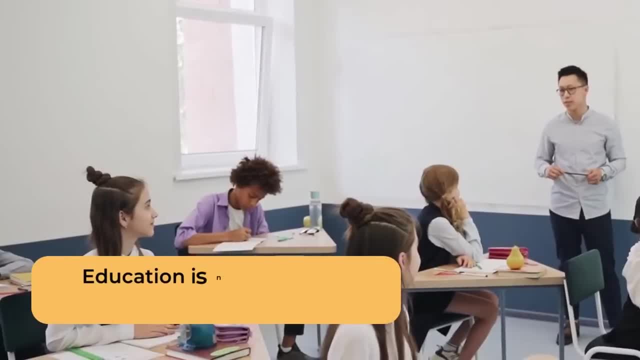 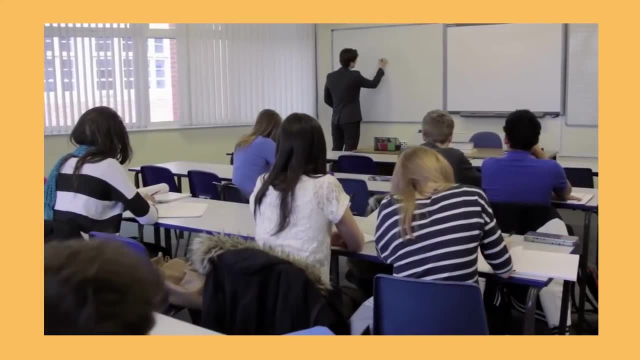 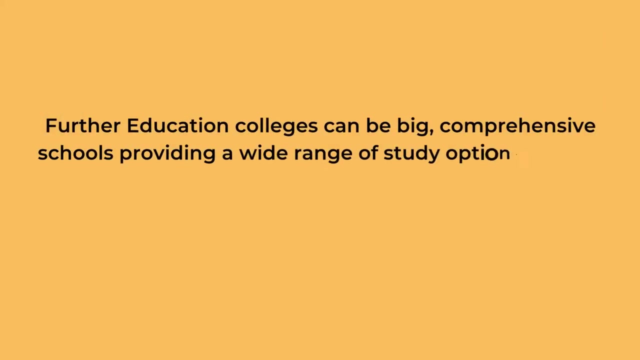 school. College education is not intended to be replaced by this program. Senior secondary education is often called pre-university education. Further Education colleges can be big comprehensive schools providing a wide range of study options, or they can be focused on a specific field of study, such as visual performing arts colleges, or agricultural or land-based. 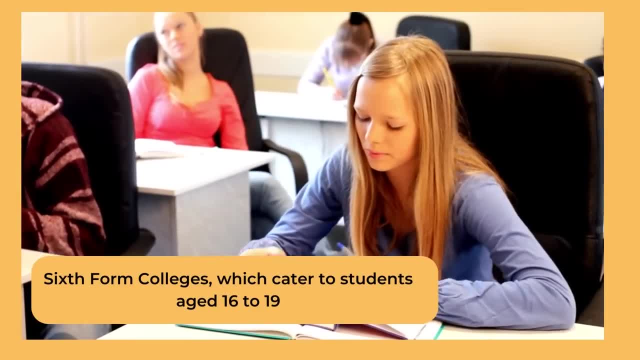 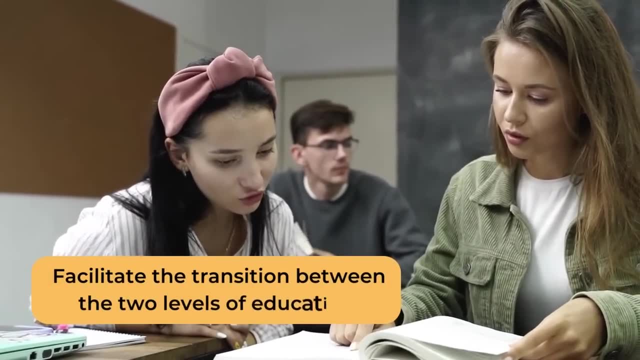 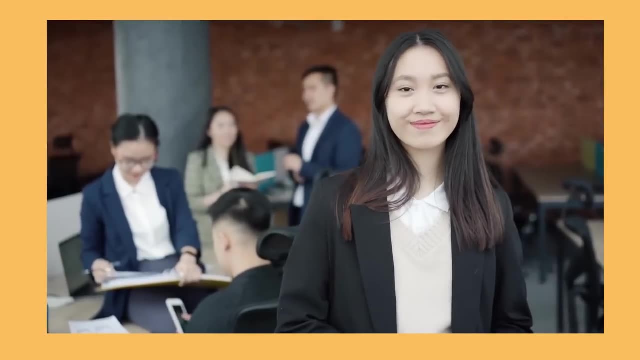 education. There are also sixth-form colleges which cater to students aged 16 to 19, and are frequently linked to secondary schools to facilitate the transition between the two levels of education- Higher Education, Undergraduate, bachelor's and postgraduate master's. and. 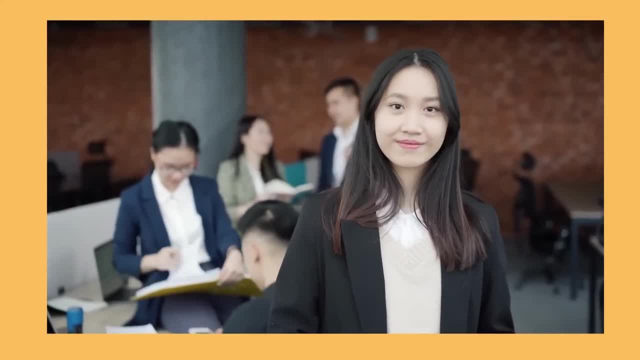 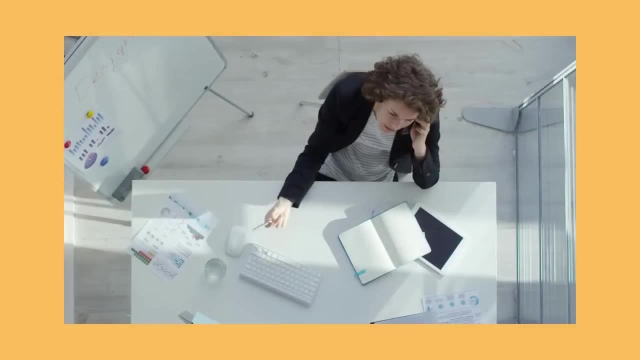 doctoral studies are both included in Higher Education. In the United Kingdom, bachelor's degrees are awarded after three years of full-time study. If a student adds a year of work experience between study semesters, known as a sandwich year, it will take four years. Five years of study are required. for professional degrees such as medicine, veterinary medicine and architecture, A master's degree may be earned in as little as a year, whereas a doctorate takes three to five years to finish An integrated master's degree.